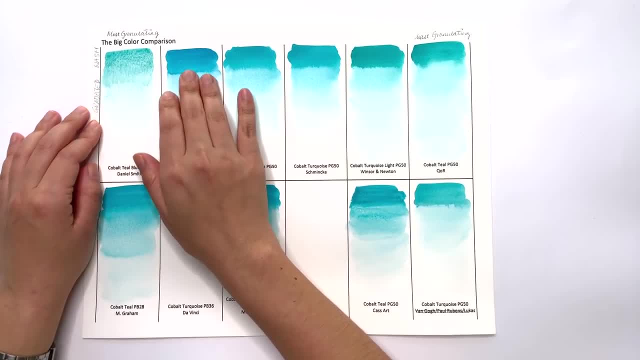 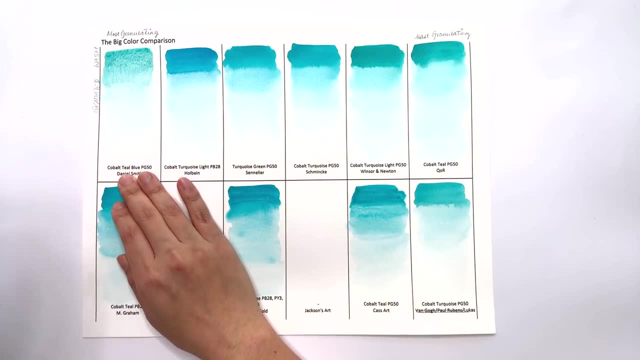 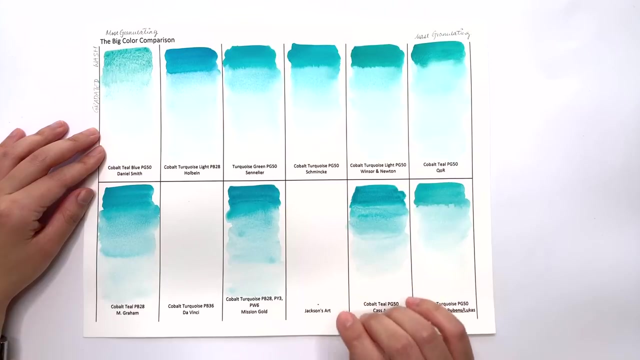 the particles rather than having a consistent looking color in the mass tone. However, it does gradate beautifully. I think it's the most beautifully gradating, evenly gradating color we've had so far in this series. All the cobalt teals and turquoises do granulate and this is on the hot press paper, so it'll be. 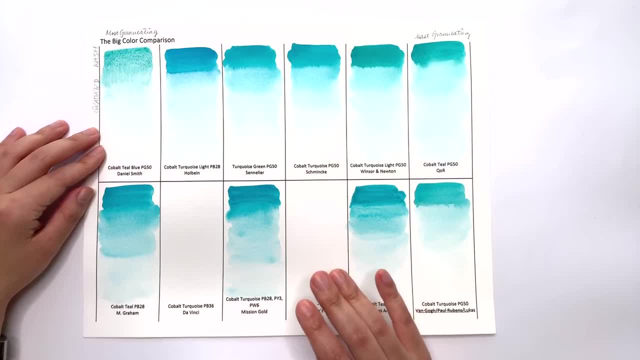 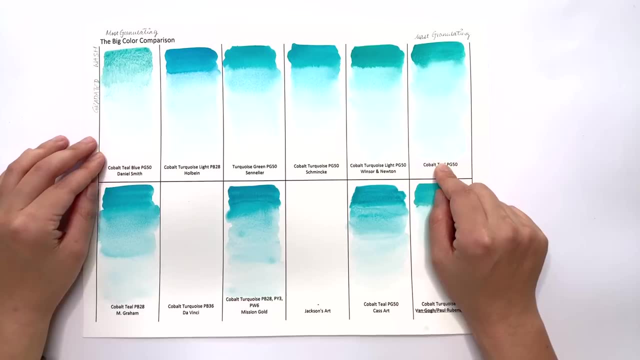 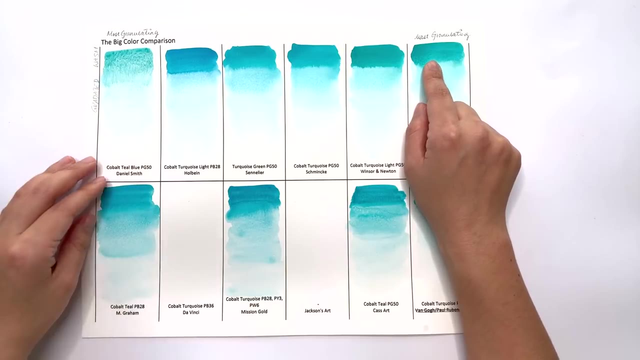 even more heavily granulating on cold press and rough paper. The least granulating of all is quartz one, Quartz one. the pigment's very, very fine and it is a huge difference, say, compared to the Daniel Smith's one. So if you are looking for a cobalt teal blue but you don't want, 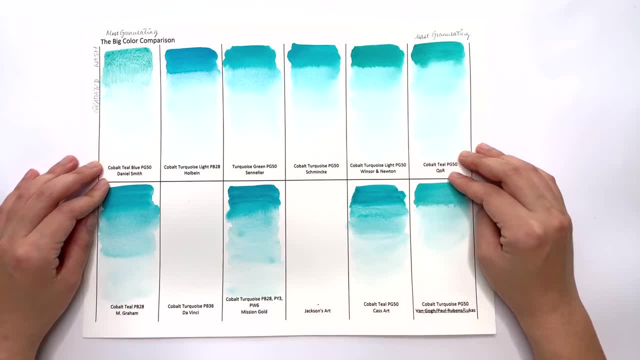 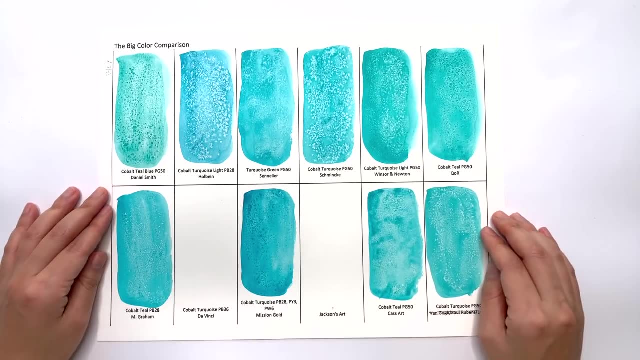 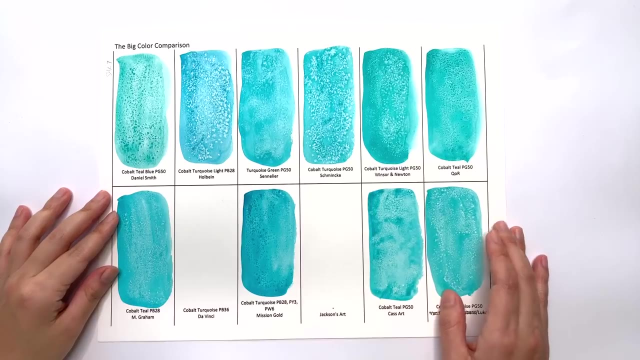 a heavy granulation, then I do recommend quartz one, And it is A lovely, lovely hue. I know color's a personal taste, but it is a really nice color. Let's now look at the salt test, And, as always, the salt tests have produced very different reactions. 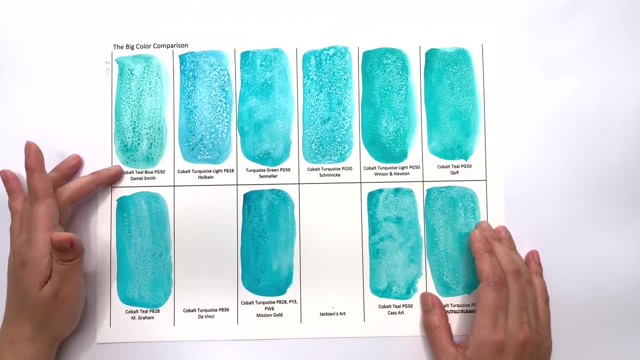 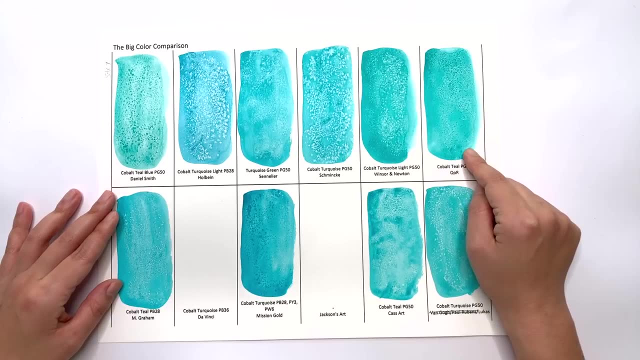 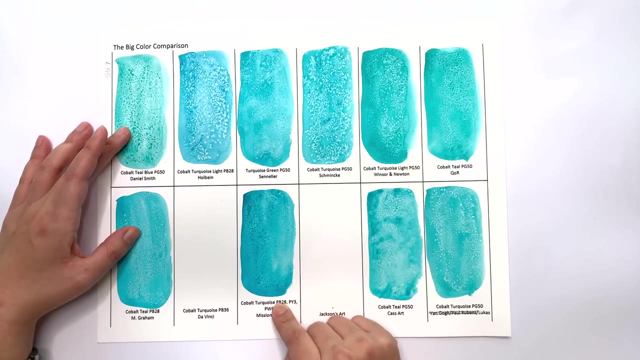 The least reactive colors of all are the Daniel Smith's, the M Graham, Mission Gold, Cass Arts and Quor one. So if you do do a lot of salt technique then I would avoid these four plus that color. The most reactive of all, I would say, is the Holbein's one and Schmincke's one. They granulate. 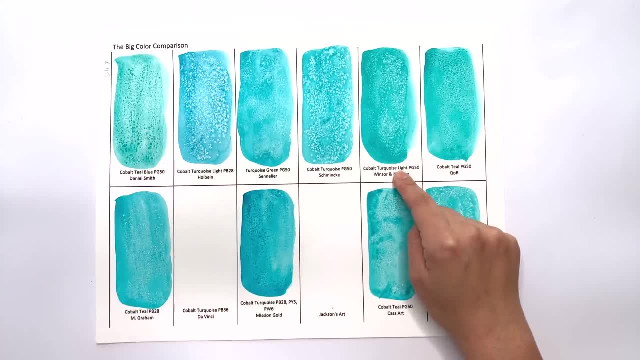 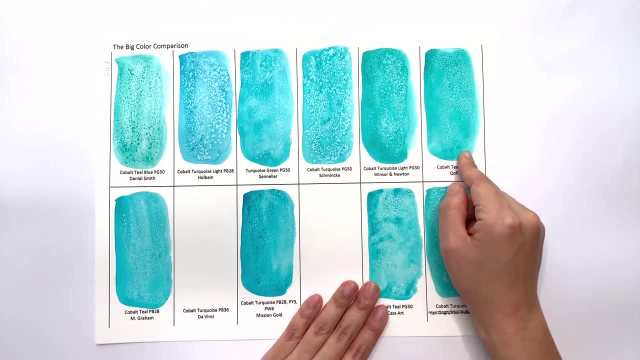 really nice, As well as the Winsor & Newton. one is medium reacting, but if you like the color of the Quor, which I really do think it's a lovely color but you want it to react to the salt, then I would. 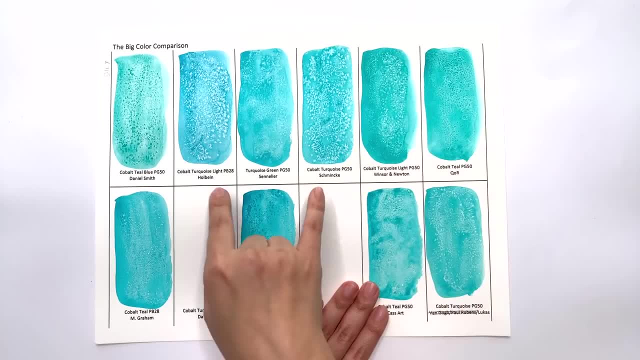 go for the Winsor & Newton one instead. But, as I say, the most reactive ones are the Holbein and Schmincke's colors. I do have to also point out the Lucas' one created beautiful patterns. It's medium reacting. 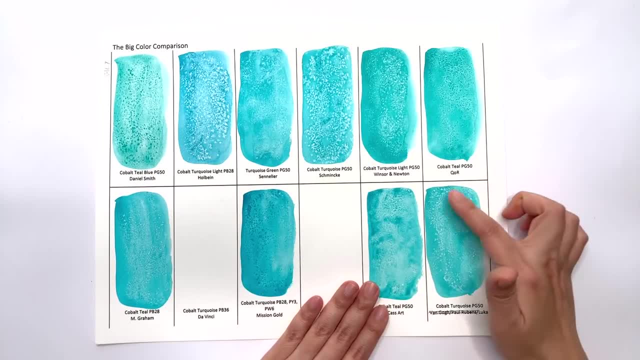 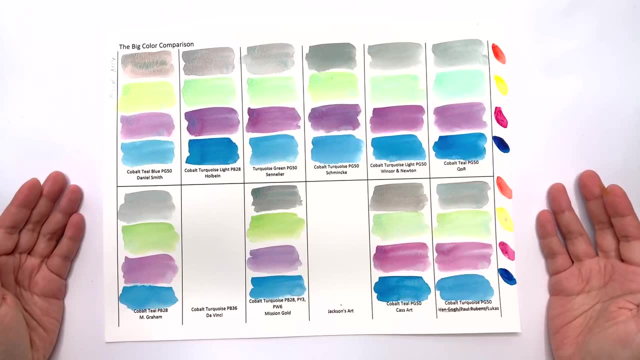 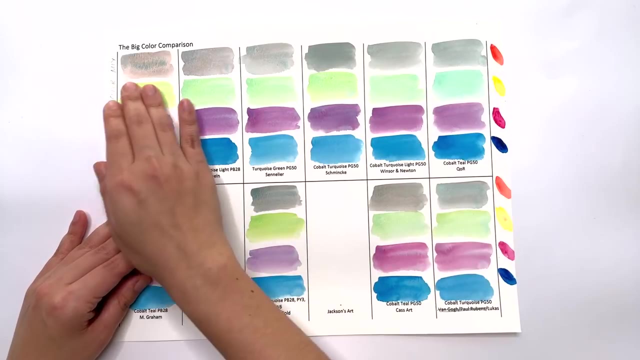 It's not as reactive as the Schmincke or the Holbein, but it is lovely, lovely pattern as well. In terms of color mixes. for the Cobalt-Tealy colors, the complementary color is the red-orange color, So I used Vermilion Hue for the complementary color to mute out the colors, as well as the usual yellow. 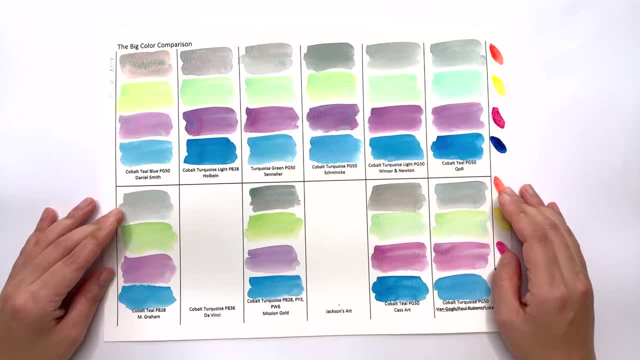 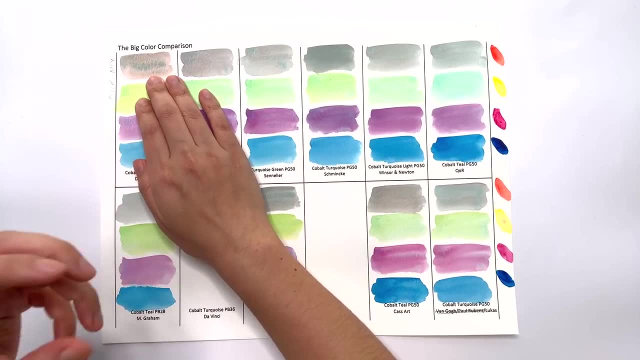 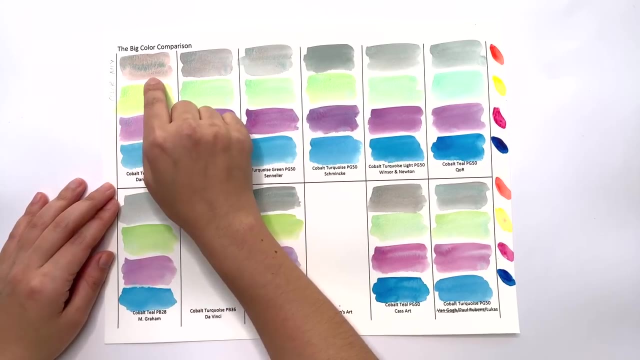 magenta and cyan colors. Not surprisingly, the Danny Smith one was the least tinting one of all. It's also the color that had color separation the most. You really see the blue pigments settling in in granulation and you really see the redness come through in the mix. and even though when you start off with a 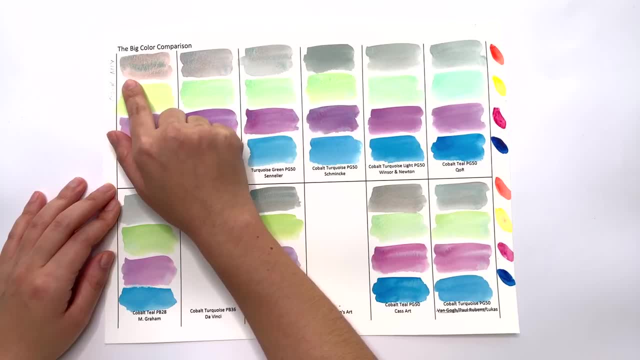 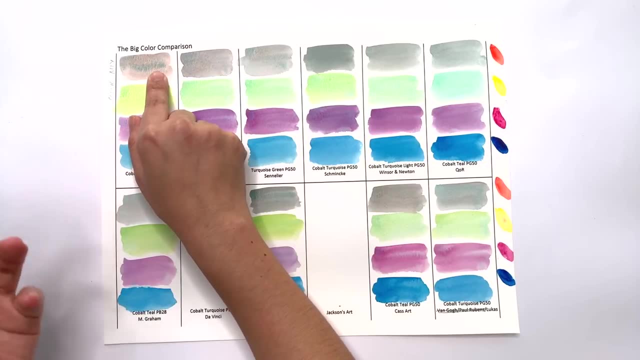 perfectly neutralized mix, you will get this color separation where the red comes through a lot compared to the other colors, as the blue pigments collect and gather together in the pits of the paper. So if you do want to be able to perfectly neutralize the cobalt teal color on your palette, then maybe 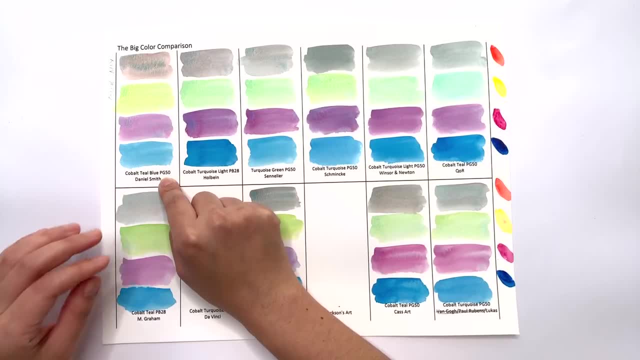 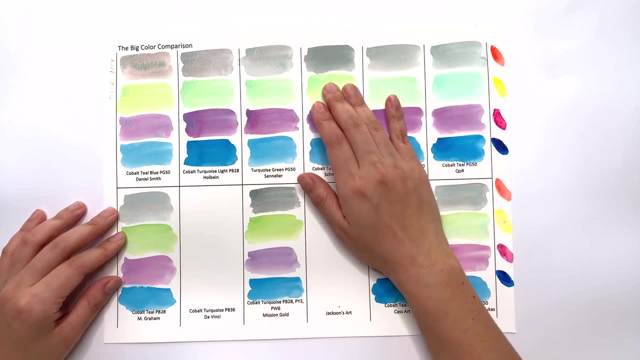 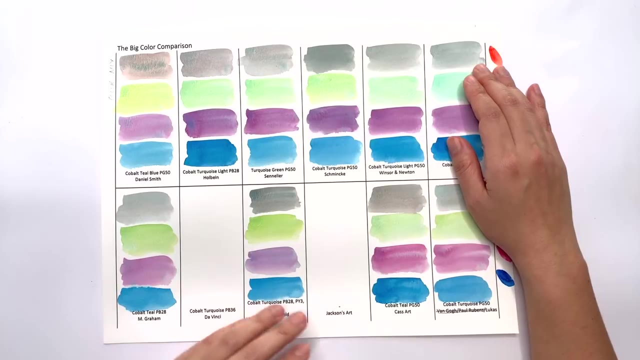 the Daniel Smith one is a little bit of a tricky choice to have, Whereas the Schmincke's one does neutralize the best out of the lot. It's very even, as well as the Quartz one, because the these colors are less granulating than the other colors, Colors that suffer from. 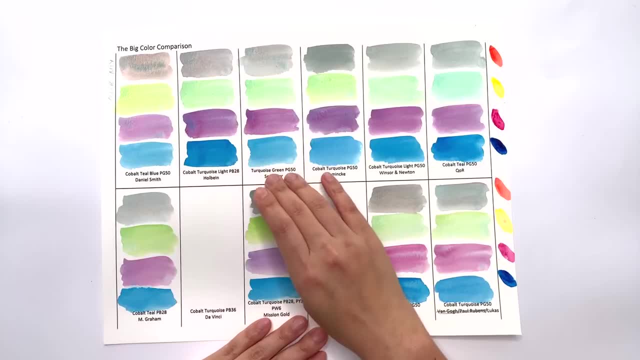 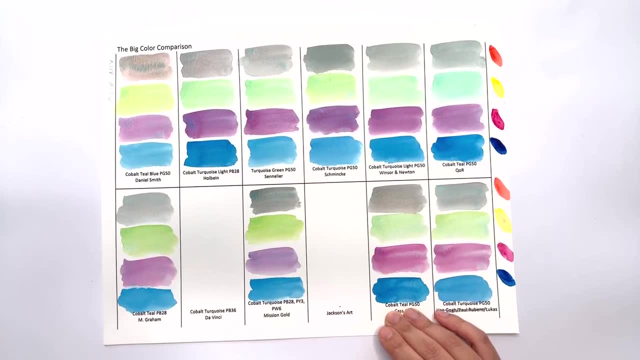 the color separation are Holbein, Sennelier, Mission Gold and Cass Art, and sometimes you do want that look. So if you do want more granulating and interesting neutrals that have a lot of textures, then I would recommend these four colors as well as Daniel Smith's one. It just depends on what you're. 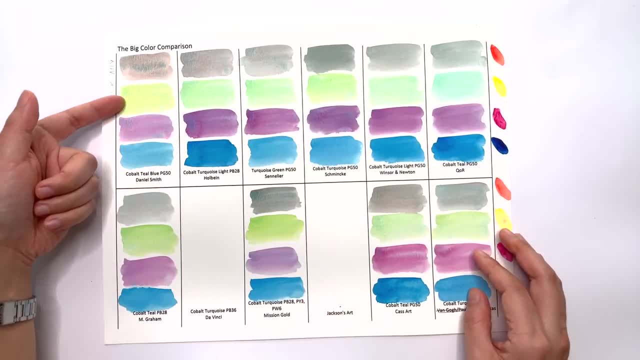 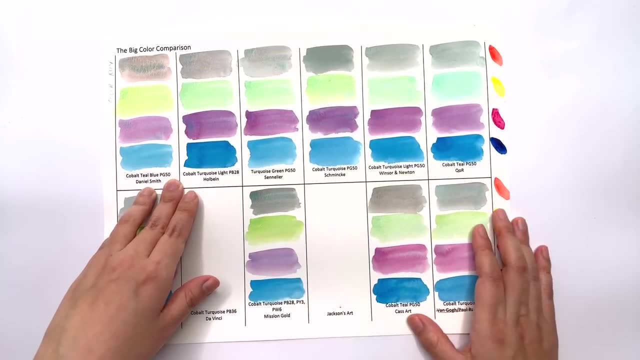 looking for. That texture does carry on on all the other colors except for the blue, because it's a blue pigment anyway, so you don't see the difference as much. but certainly mixing it with the yellow and magenta's, you see lovely, lovely color separations. 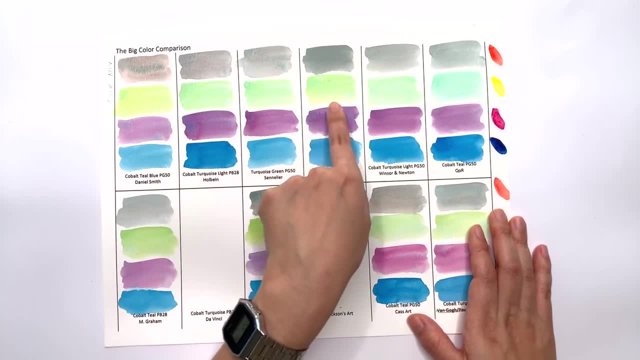 here, here, here, as well as the Schmincke's, one has this lovely, lovely green color that separates, which is interesting, considering the neutralized color was really well blended. So, in terms of choosing which Cobalt Teal to go for when it comes to color mixes, 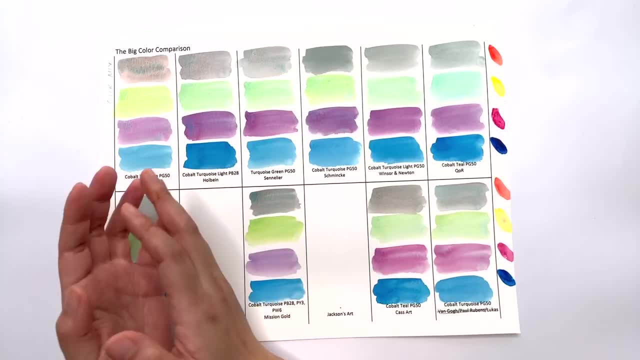 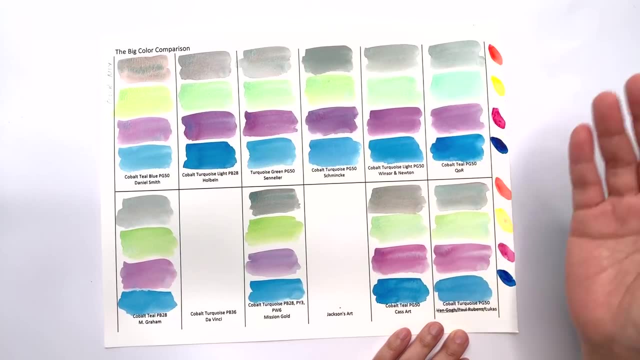 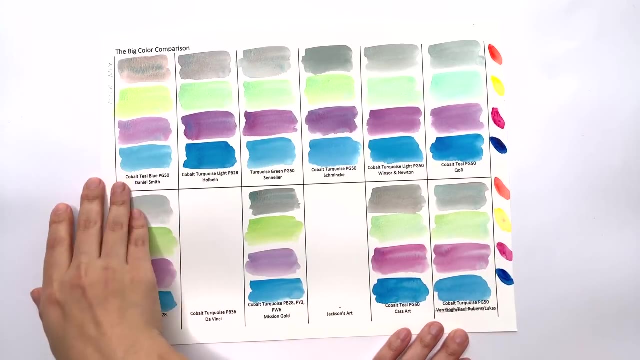 it just really depends on whether you want a lot of texture in your color mixes or if you want an even color. If you want to do even colors, go for something like the Quartz, even the Lucas one. They blend really, really beautifully. and if you want to go for more texture, the extreme version is the Daniel Smith. 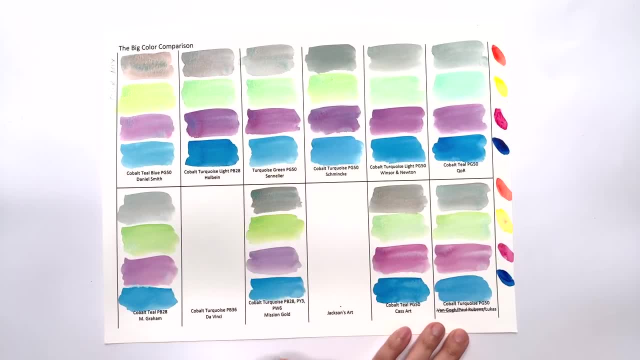 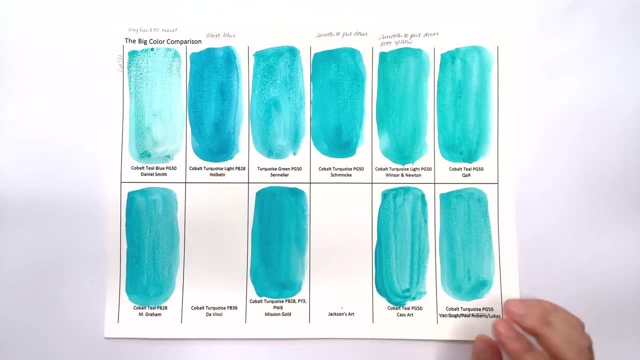 otherwise go for something like the Holbein, Sennelier and Mission Gold. The other colors are somewhere in the middle. So which color would I go for? Well, hue wise, I really like the Quartz. It's a lovely teal color. It's what I would think. 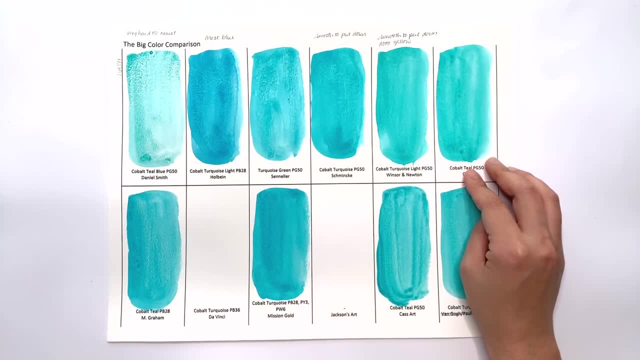 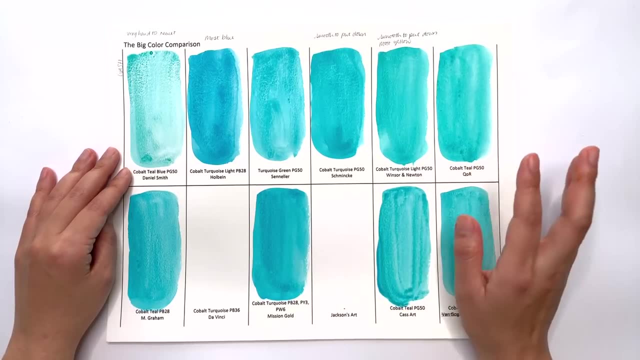 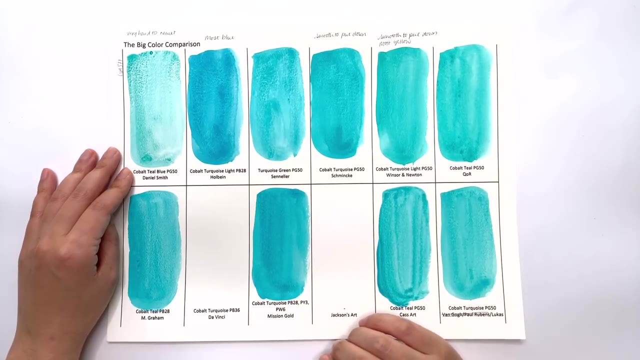 of when I think of teal color. However, for me personally, the Cobalt in my mind should granulate quite heavily, and so for the Quartz one to not granulate hardly at all is not what I'm personally looking for from a Cobalt mix. If you want a non-granulating Cobalt color, it might be that you want a non-granulating. 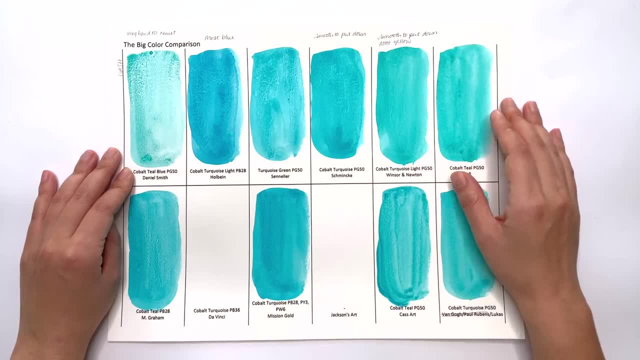 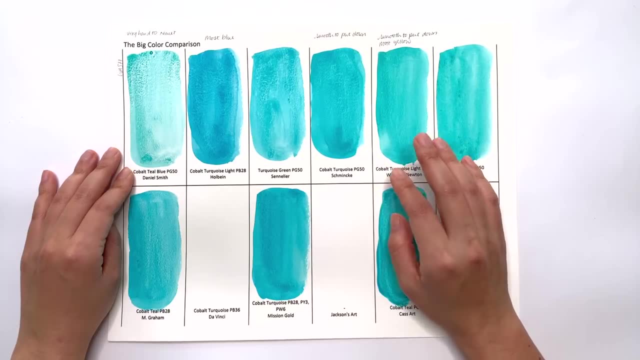 Cobalt color, in which case the Quartz is perfect. If you do love the color but a little bit strapped for cash, then go for the Winsor & Newton's one, because it does go down smoothly and it's very similar in hue, but it does have a little bit. 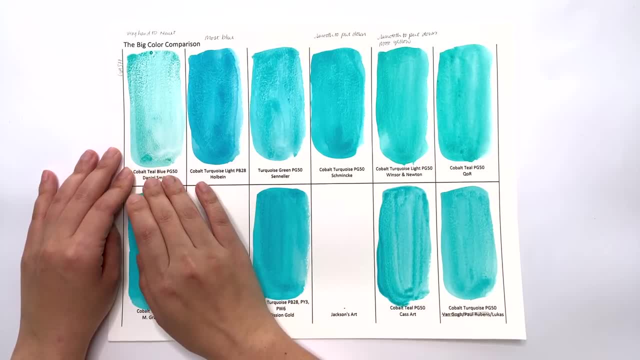 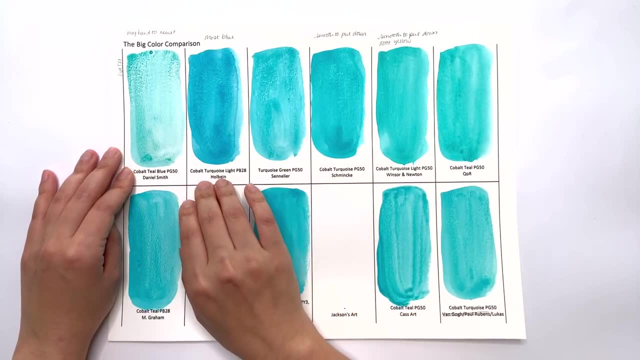 more granulation than the Quartz one. I would say that the Daniel Smith one is a little bit too granulating for me. I want something in the middle, and in this case I would say that the Holbein's one is a little bit too blue. So I'm definitely. 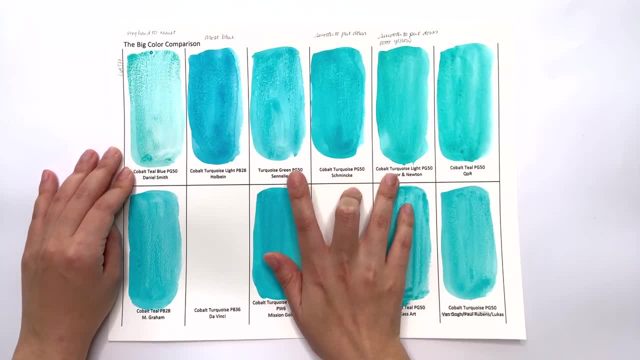 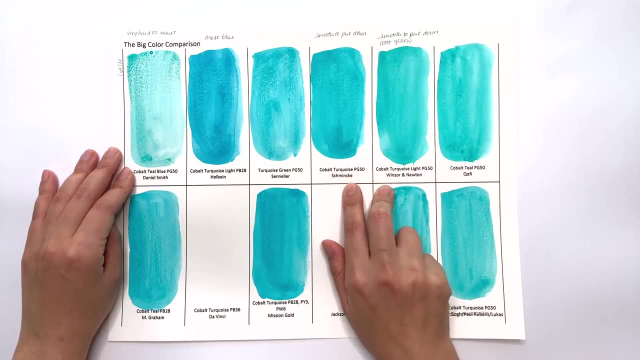 looking for something in between here. I'm still not that comfortable with Sennelier, so I would say I would go for somewhere between the Schmincke's one and Winsor & Newton's one for the hue and the medium amount of granulating that. 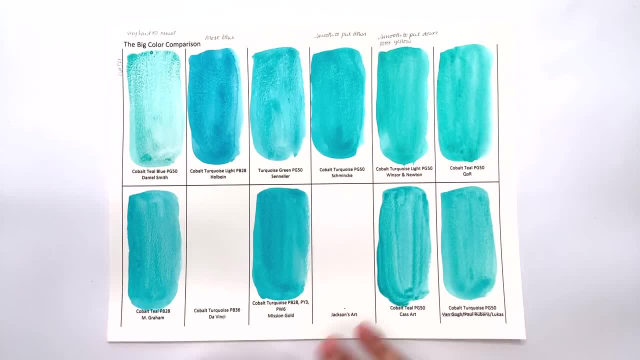 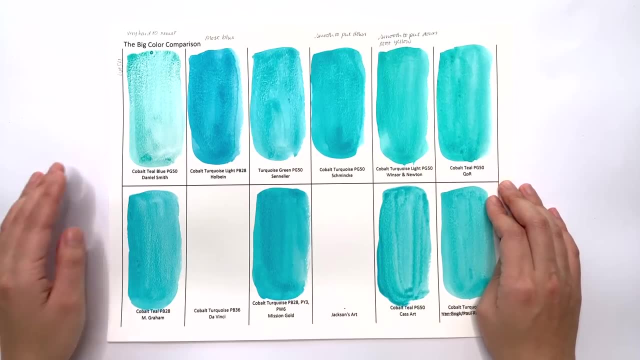 you get. I think it's really nice balance. So which one was your favorite? Did you start off with one favorite color and moved on to a different favorite color By watching this episode? If so, do let me know in the comments down below. It's so. 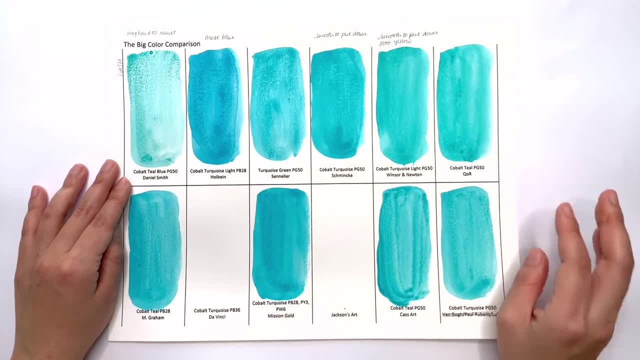 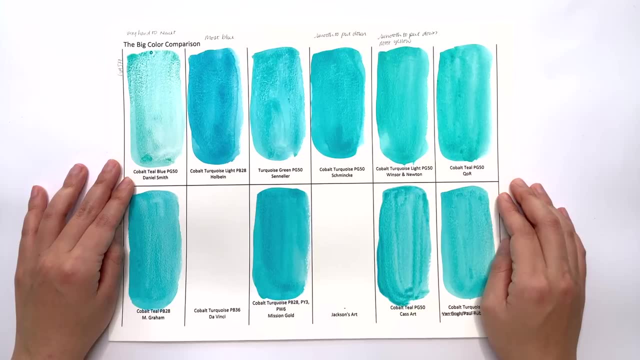 interesting to hear how people have changed their minds about what their favorite color is or want to try a new color by a new brand that they haven't tried through watching this series. So thank you so much for all your comments. If this video was useful and interesting to you, then please do give it a thumbs. 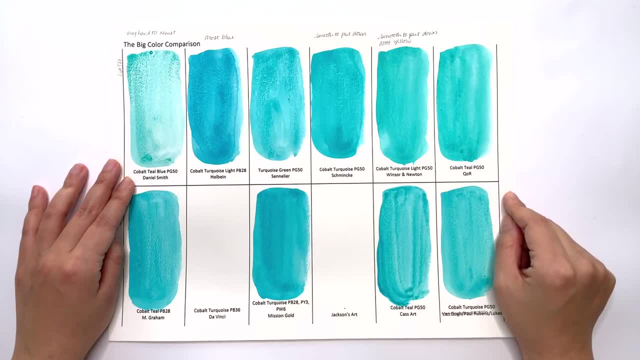 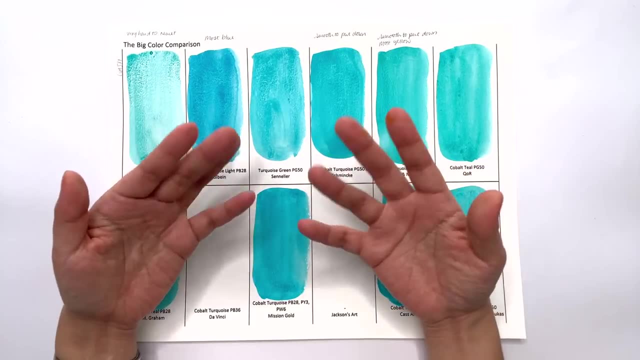 up Subscribe to this channel if you haven't done so already. Thank you so much for watching and I'll see you in the next one, Bye. Thank you for watching this video and I will see you in the next episode. Bye.